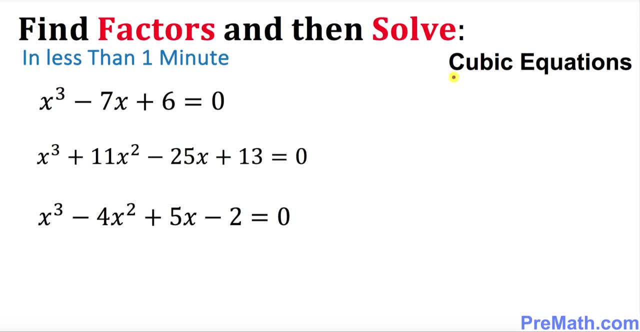 hello again, everyone. in this video tutorial I am going to show you a super easy way to find factors and then solve these given cubic equations. and the very first thing before we get started is to see whether these cubic equations are in standard form. and, by the way, the cubic standard form looks like this one, as you. 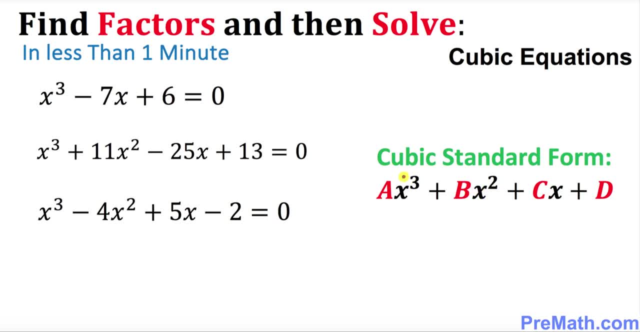 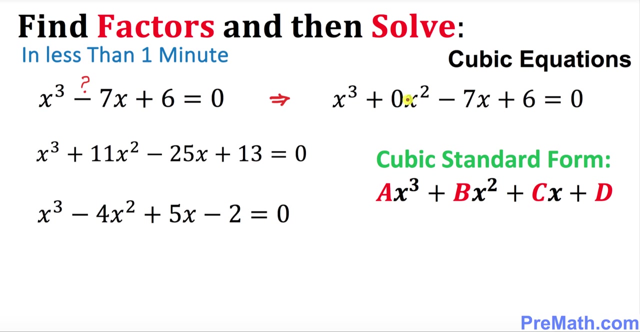 can see over here. if I compare this one with our given cubic equations, then we can see that obviously X, power 2 is missing in this very first cubic equation. so this cubic equation could be written as zero time, that missing term and everything is same. now let's get started. 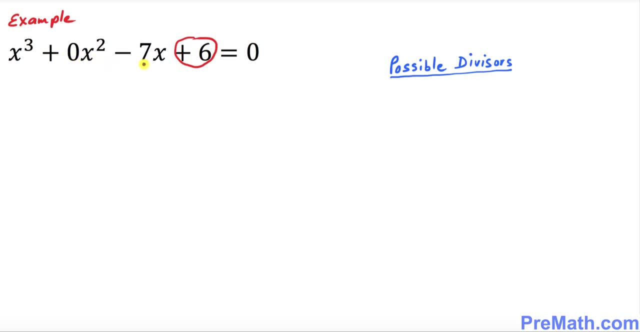 with the very first example. it is right up here this cubic equation. I want you to focus on the very last number, that is positive 6. so now we're going to see what are the possible divisors for positive 6. obviously that's going to be positive and negative: 1. positive negative 2. positive negative 3. 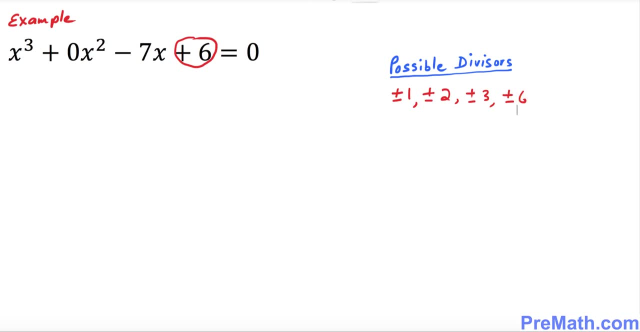 positive, negative 6. so the next step is: I want you to look at this cubic equation. since the highest degree is 3, so we must have at most 3 solutions. so we're going to pick three feasible numbers among these one the possible divisors that if you add them, that's going to give you this number 0, and if 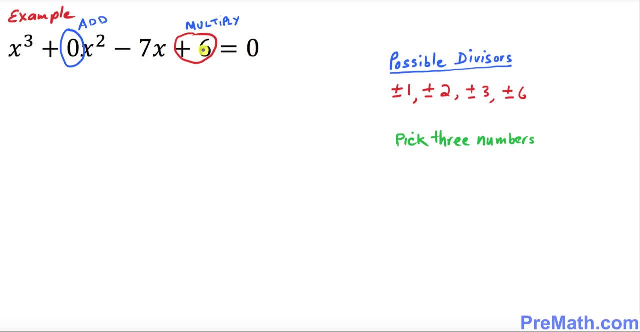 you multiply them, that's going to give you this positive 6. so now ask yourself: what are those going to be, those numbers among these one? so that's not, that's not really hard. you pick negative 1, negative 2 and 3. okay, go ahead and multiply them. 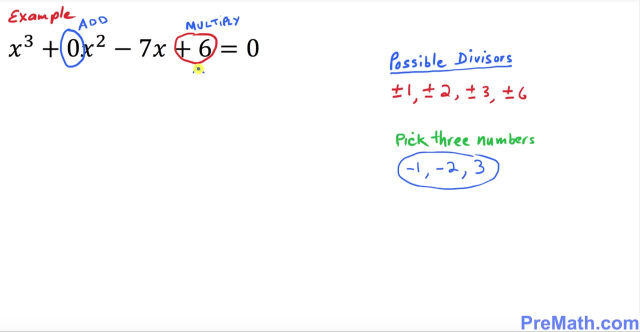 out, isn't it? that's gonna give you positive 6. okay, good, and how about if you add them? that's going to give you, for sure, 0. so thus, our factor is going to be simply: you just put in a parenthesis X and then minus 1. you just put down minus 1. 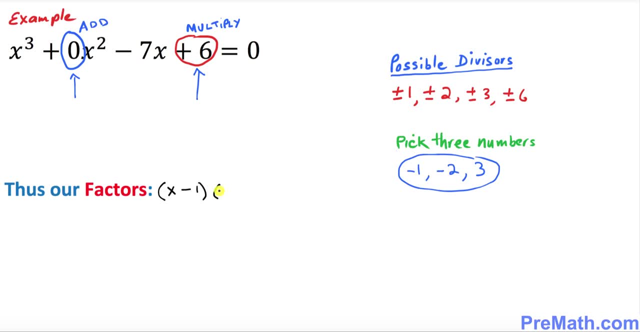 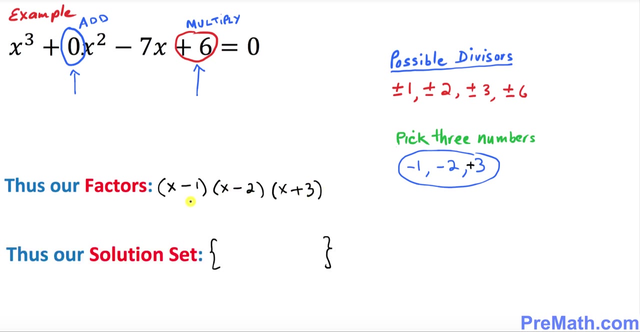 whatever that's number is, and then X minus 2, and then X, and this is a positive 3. so this, this is your factors and finally, our solution set is gonna be: whatever you got these factors, you just change the signs. so this negative 1 become positive 1, this negative 2 become. 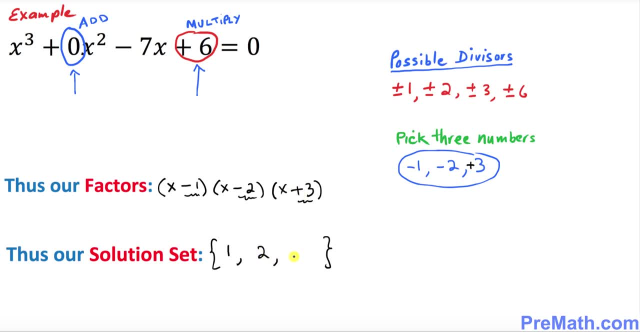 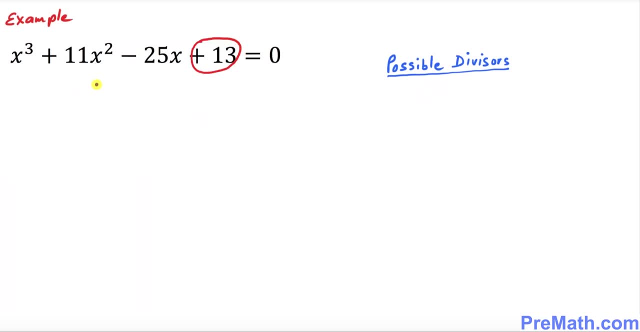 positive 2, and this positive become positive 3, become negative 3, and that is our answer. and now we're gonna look at the next example, and over here I want you to focus on this very last number, which is positive 13. so what are the possible divisors for this one? obviously, 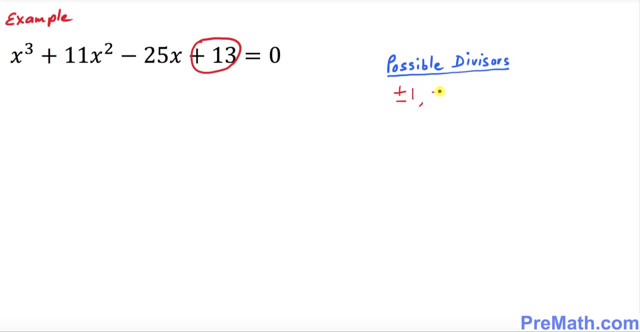 they are going to be a positive negative 1 and positive negative 13. and now the next step is we are going to pick any three feasible number among these divisors. if we add them, it's supposed to come out to be positive 11, and if we multiply them, this should be positive 13. so those numbers gonna be: 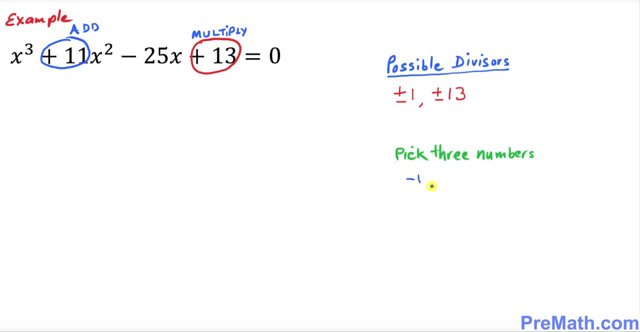 pretty simple, isn't it? negative 1, negative 1 and 13. now I want you to go ahead and multiply this thing. obviously it's gonna give you positive 13, and if you add them, that is gonna give you positive 11. thus our factors for this given cubic equation turns out to be: you just put down. 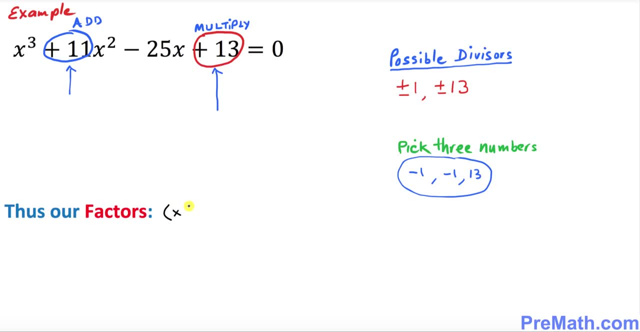 parentheses and then x over. here you have a first one is negative 1, you put down minus 1. the next one is minus 1 again, put down negative 1 again. and the next one, this is positive 13, so the X plus 13. so these are your factors, and 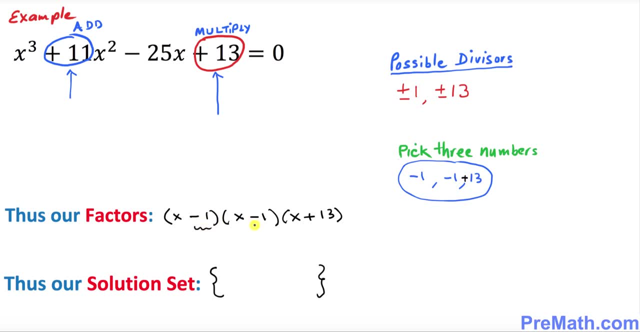 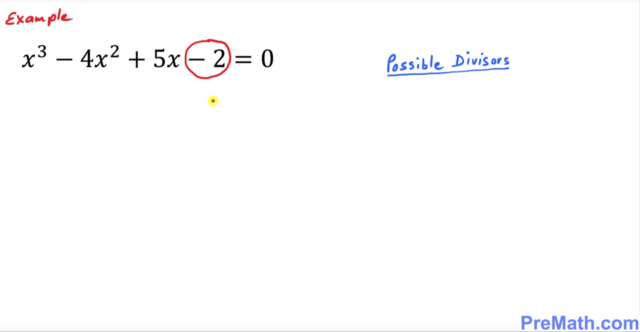 our solution set is gonna be: you got these factors, you just change the sign numbers. so sign negative one become positive one, switch this sign become positive one and this become negative. 13 and that is your answer. and finally, let's look at this last example over here, over here, what is the last? as you can see, 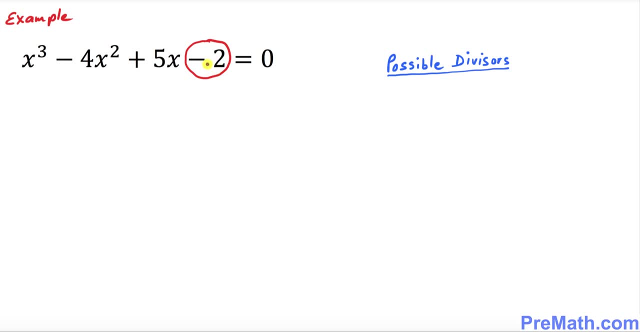 the last number over here in this equation is negative two. now ask yourself what are the possible divisors for this number? and obviously that's going to be positive, negative one and positive negative two. and in this step i want you to pick any three numbers from these possible. 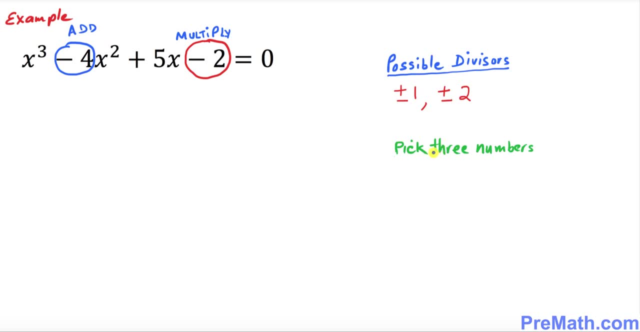 divisors that are going to work for us. if you multiply them, they should give us negative two, and if you add those three numbers, that should add up to negative four. so the numbers are going to be, if you try them, negative one, negative one and negative two. okay, so those are the one, and now what i want you to do is go ahead and multiply. 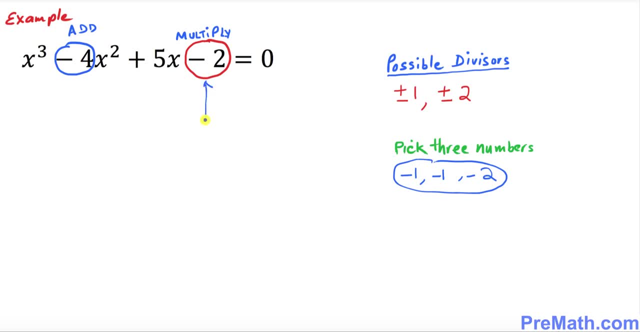 these numbers and you can see that we're going to get negative two, and if you add them up, that's going to give you negative four. thus, our factor is going to be simply: you just put down these x minus whatever. this number is negative one times once again, the next one is negative one again, and finally, x minus two, and these are your.